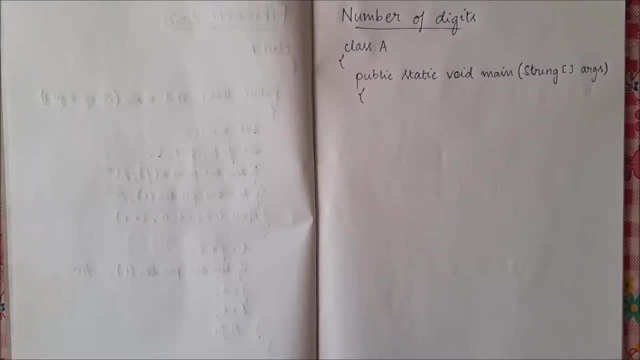 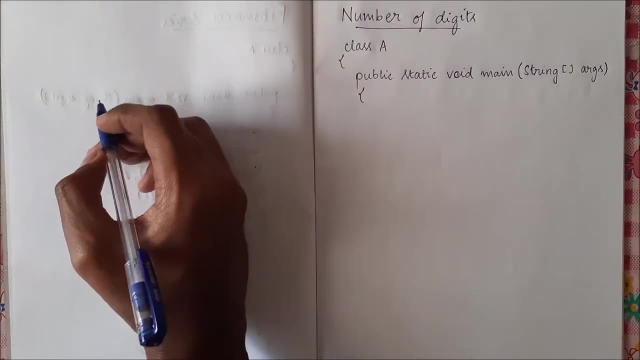 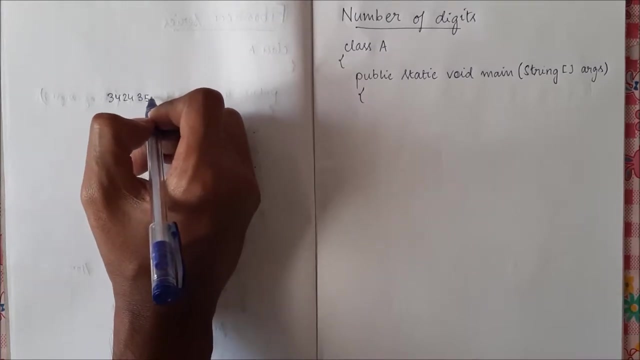 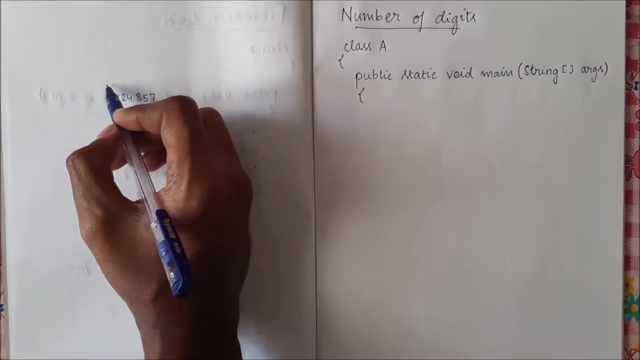 Hello, in this program let us learn how to find or how to count the number of digits in a given number. So let us say we have a number, So we have to count how many digits this number has. So if we manually count 1,, 2,, 3,, 4,, 5,, 6,, 7.. 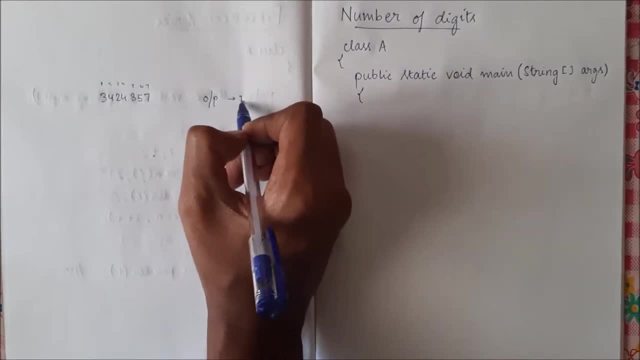 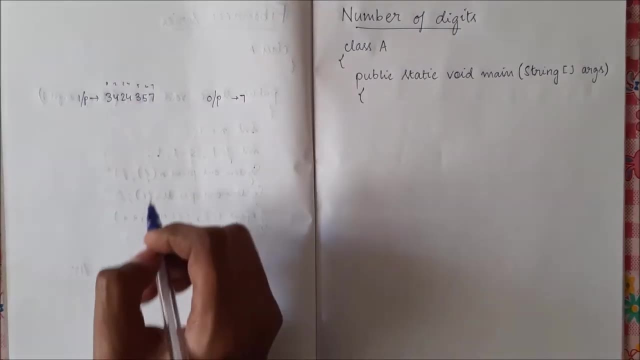 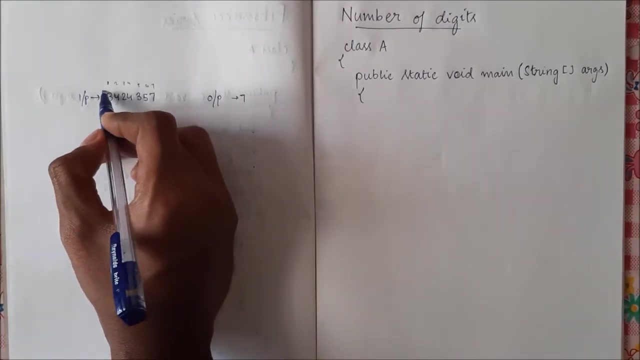 So our output should be 7 for this input. So how do we count the number of digits? So a simple logic is: we will divide the given number by 10.. So if we once divided by 10, since it is an integer number, if we divide this is an integer number. 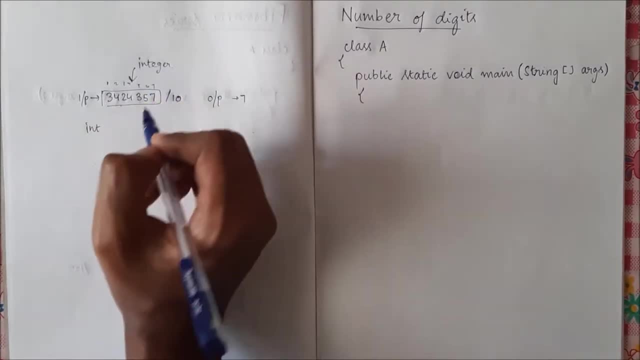 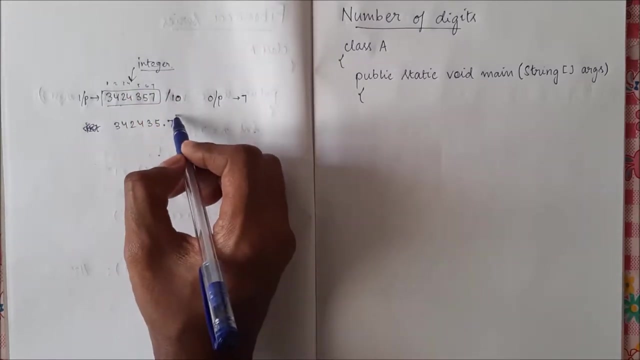 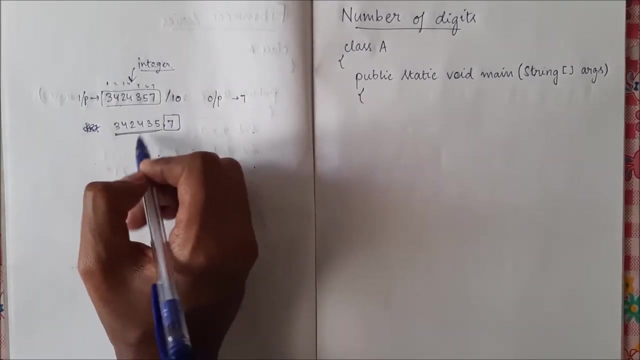 So if we divide it by 10, we will get. this is the actual value, But since it is an integer, it will not consider this decimal part. So our output will be this if we divide by 10.. Next time when we divide this number, 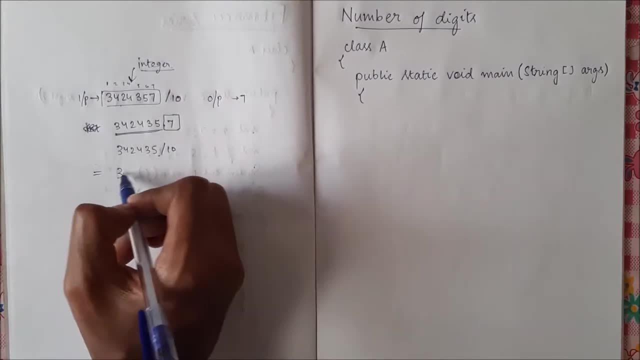 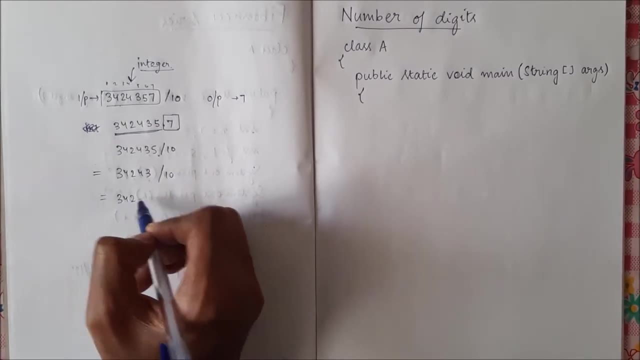 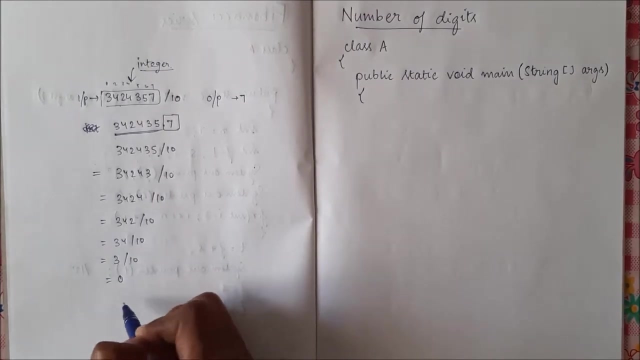 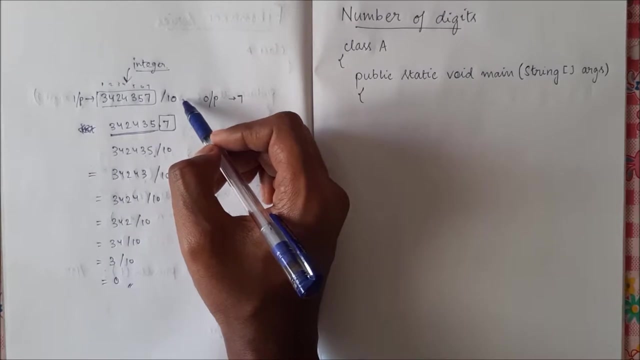 by 10.. It will result in again, you, divided by 10, will become three, four. so in this way you have to keep on dividing, keep on dividing until we get 0. So once we get 0, we are have to stop our loop. so we can see the count as the number of times we have divided it. 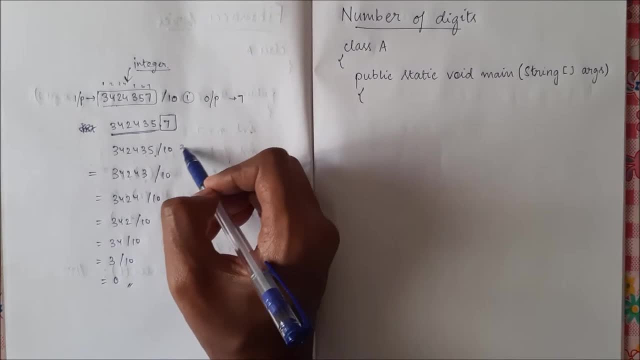 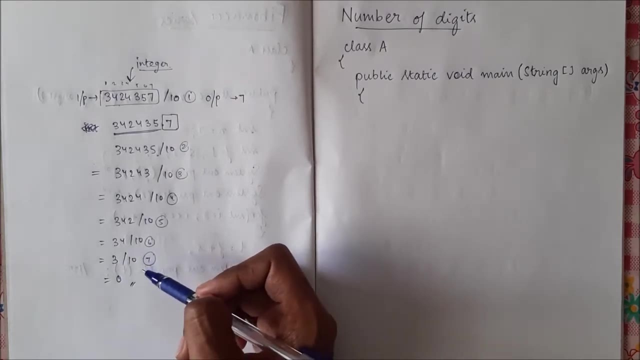 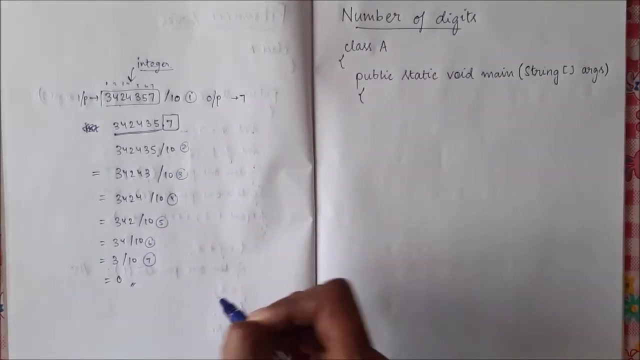 by 10, so 1, 2, 3, 4, 5, 6, 7. so we were able to divide the number by 10, 7 number of times. so our output is 7. so let us see how to do it. so when should we end our loop? when our 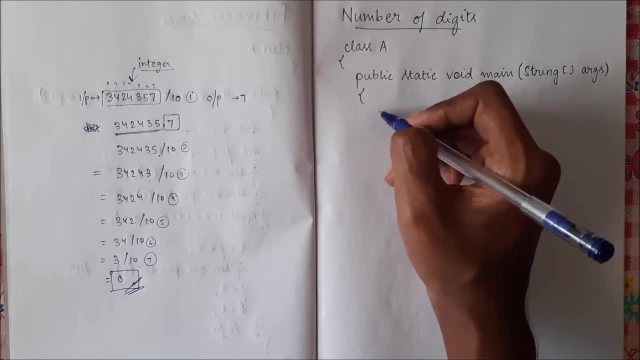 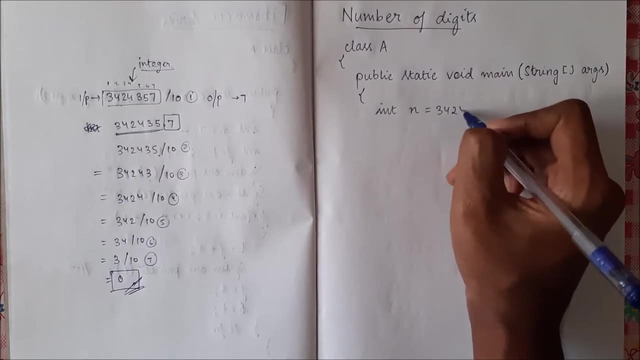 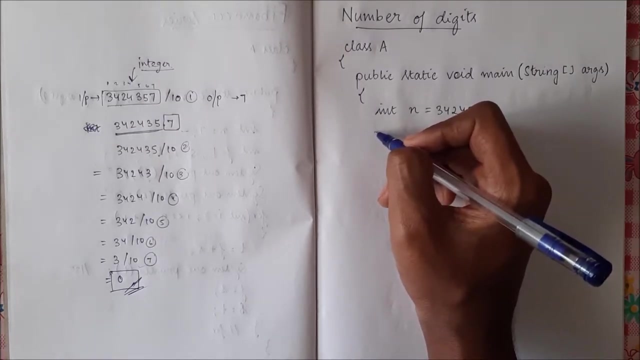 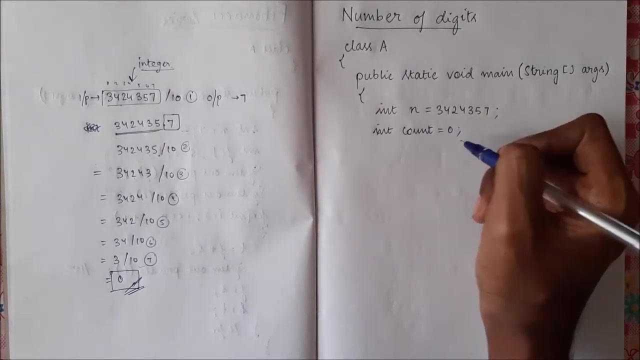 result becomes 0. so let me first create a variable called n. our n will have the input value. let us let us create a. let us create one more variable, count, which is initially 0, and we will use this variable to count how many digits we have. 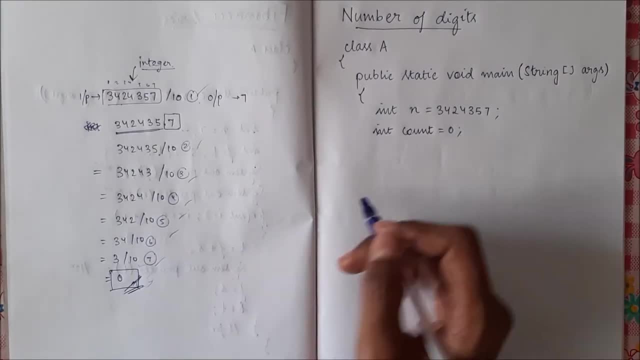 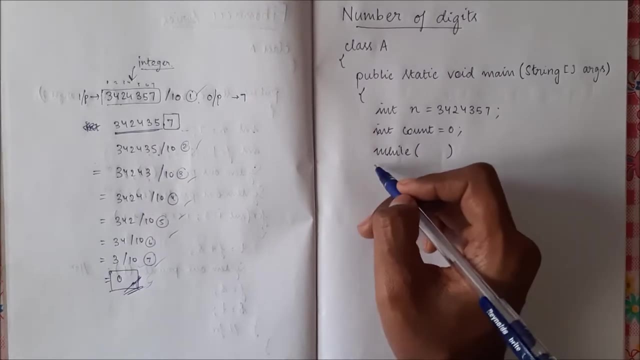 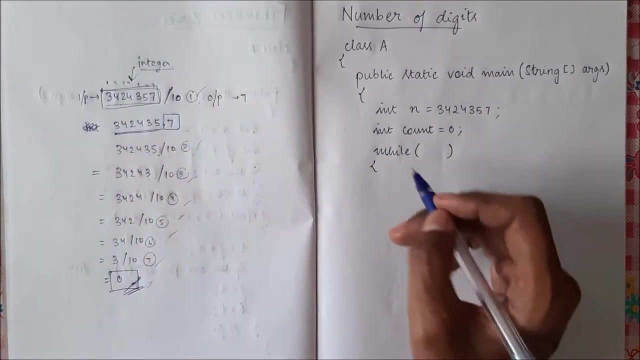 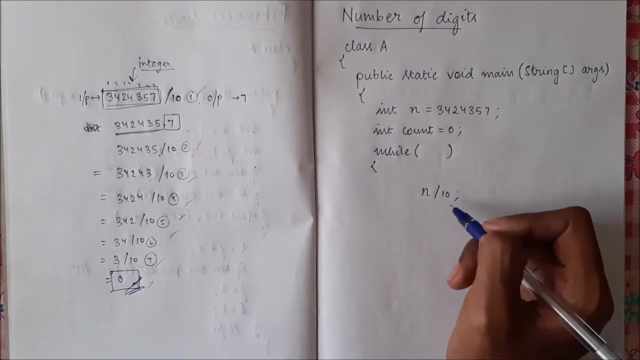 so now, with this base condition, we'll write a while loop. i'll put the condition later. okay, so what this is: n. we are dividing the n by 10, so i'll write n by 10.. now this: i will store it back to n. so initially, what this statement will do is it will divide. 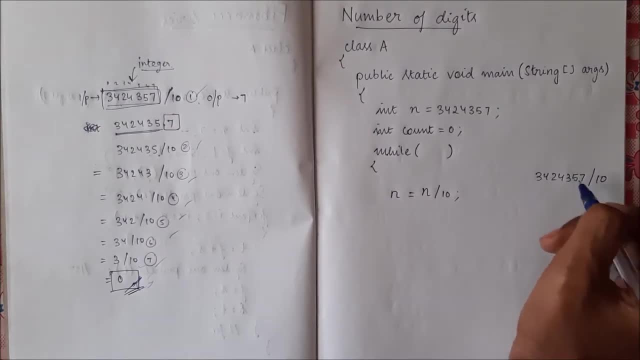 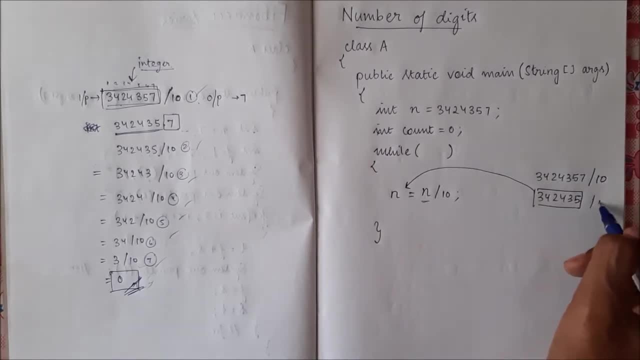 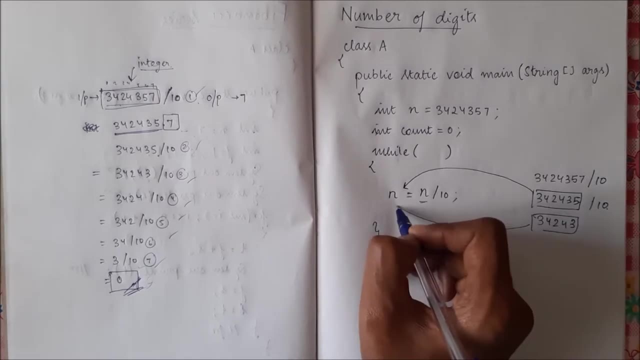 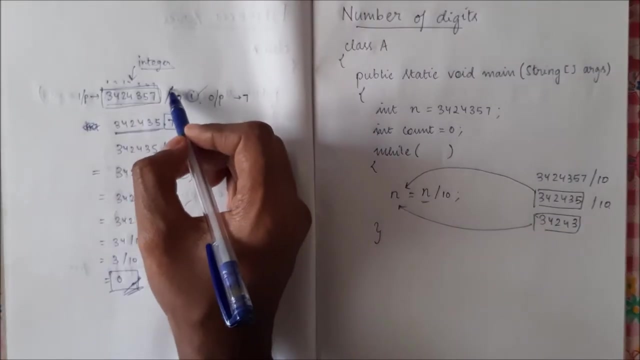 this n is 3, 4, 2, 4, 3, 5. again it will be divided by 10. the result will be this: this will be again stored to this, so this way it will keep on iterating. after doing this once, when we divide it by 10, we are doing count once. so i'll say: 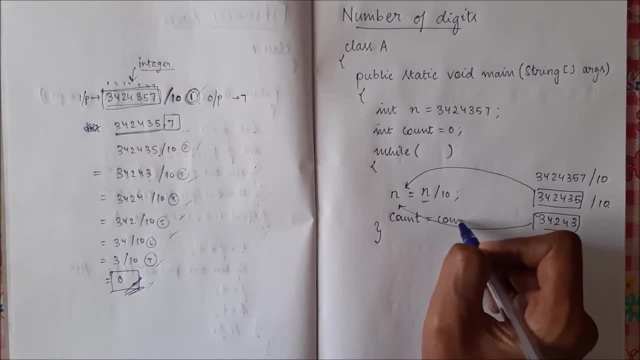 count equal to count plus 1 and when it should end. see, first n was this, then we divided by 10. it became like one last digit, first remote. now again this difference was removed. again we divide, this digit will be gone, then again we'll divide and finally it will arrive to zero. so finally n will become zero. so when n is,